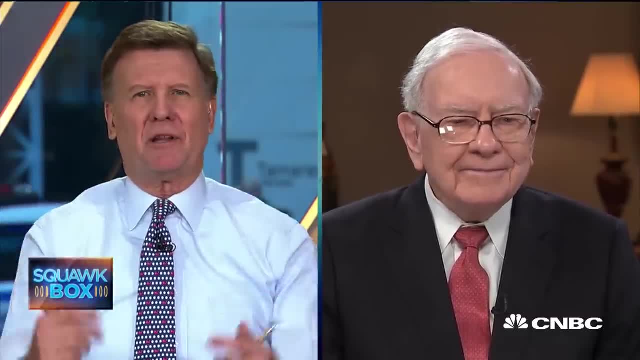 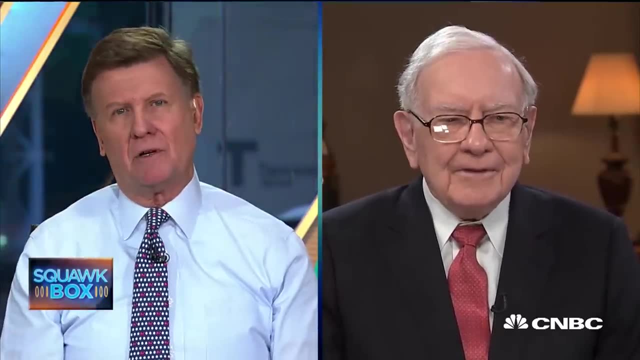 I know, All right, And you can tell it to switch. You can verbally tell it to. you know, switch to something else. Switch to Squawk Box, for example, which is apparently one of the most common verbal, or switch from Squawk Box. 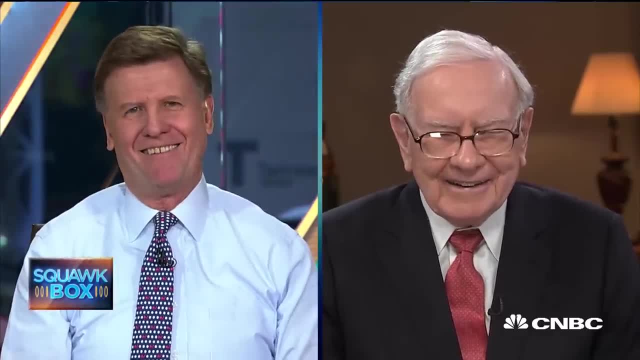 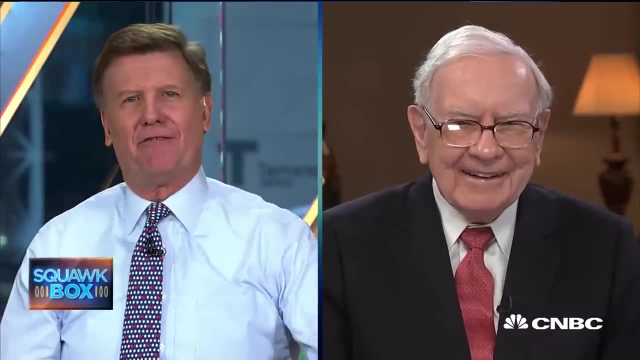 No, I'm kidding. Anyway, go on. All right, I watch you on an 85-inch screen. Oh my God, I know We don't pay our makeup people enough. I know, No, we don't Wow. 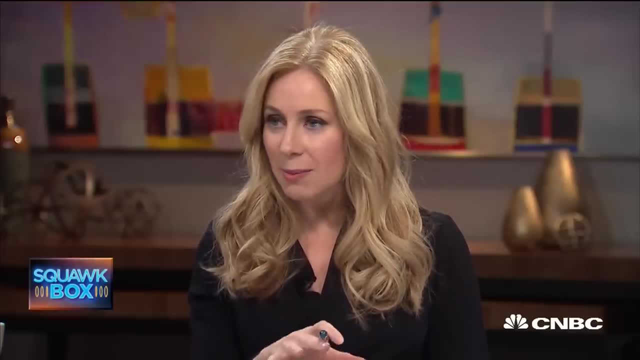 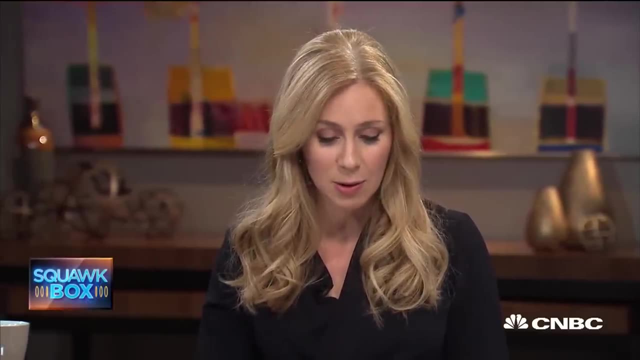 All right, Warren. we want to take this part of the show and get some questions from some of the viewers who have been writing in and sending things in too. A lot of these are people who read your annual letter and have additional questions about Berkshire too. 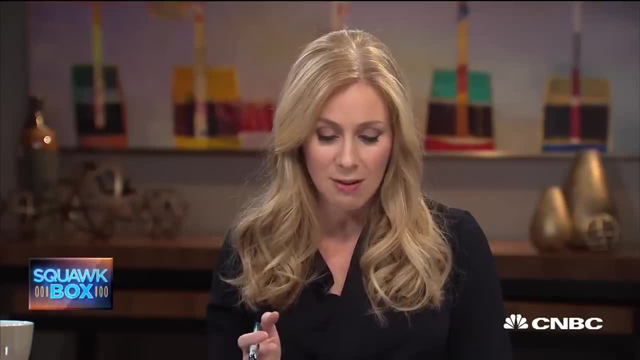 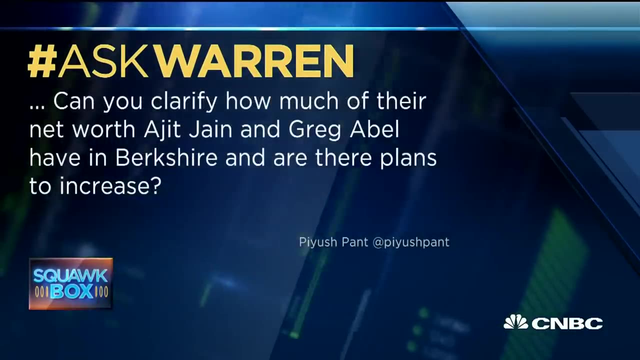 First one comes from Piyush Pant, who says: Both you and Charlie have the vast majority of your net worth in Berkshire stock, which means that you share the pain if things go south. Can you clarify how much of their net worth Ajit and Greg Abel have in Berkshire and are there plans to increase? 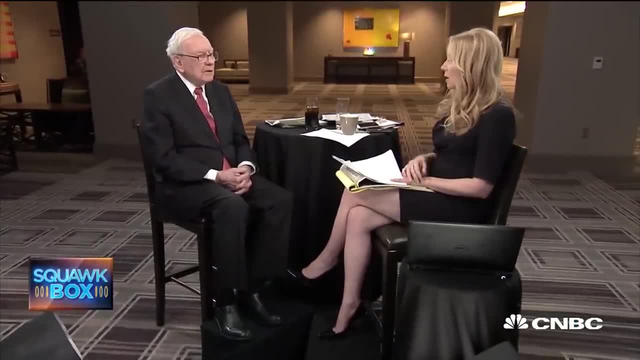 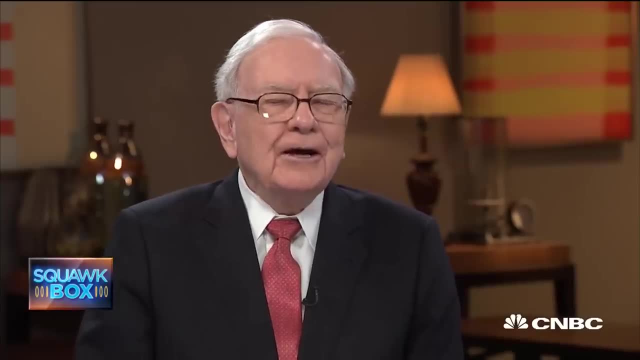 Now they did disclose their holdings as directors in terms of Berkshire, But that doesn't really tell about their net worth. Yeah Well, I've never asked them about their net worth. That's their business. But Ajit obviously has a very substantial investment. 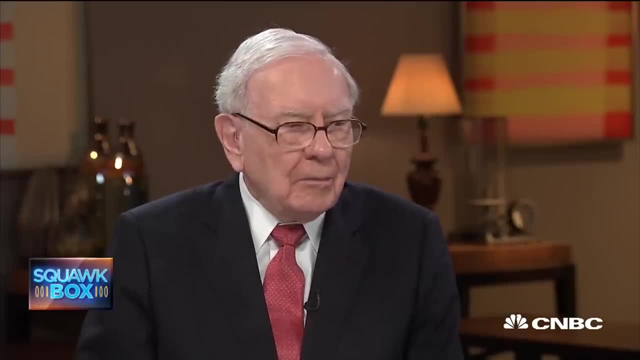 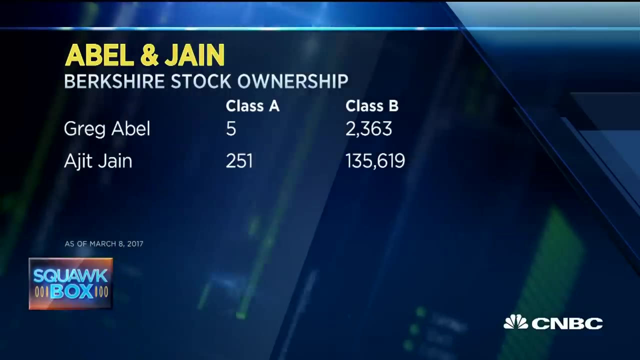 He's bought every share of that in the open market And he came into my office in 1986 on a Saturday And I don't think he had very much net worth at that time And he's just bought Berkshire as he's gone along. 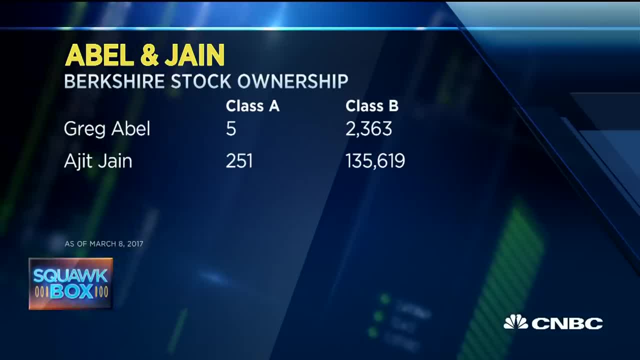 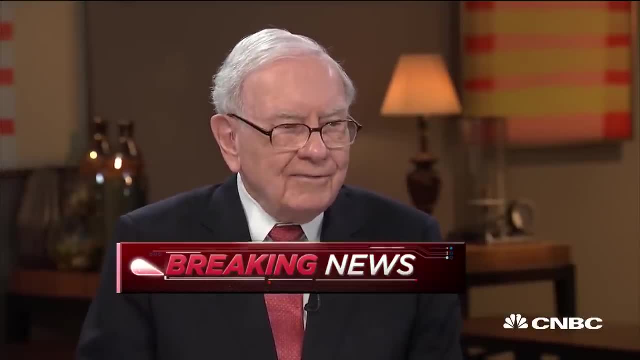 And Greg has been with MidAmerican Energy. He's now Berkshire Energy for well over 20 years And his net worth is virtually 100% in Berkshire. I don't know that it's 100% because I don't know what he has outside. 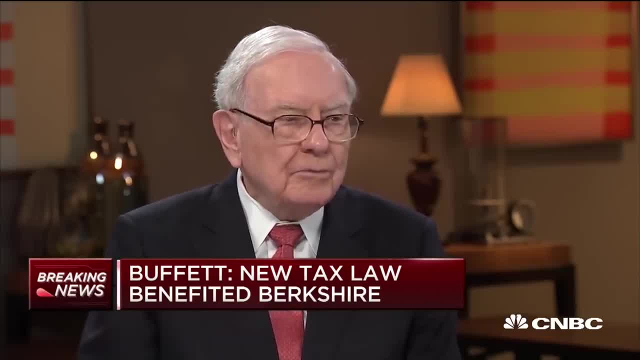 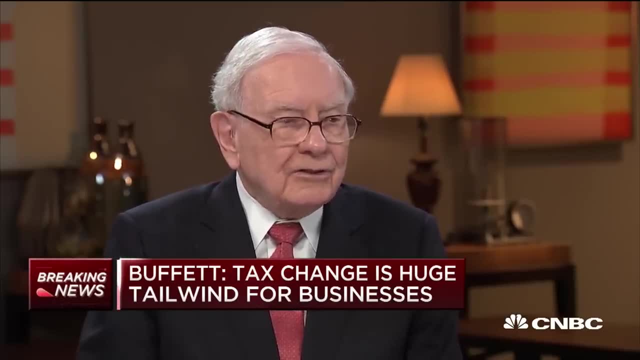 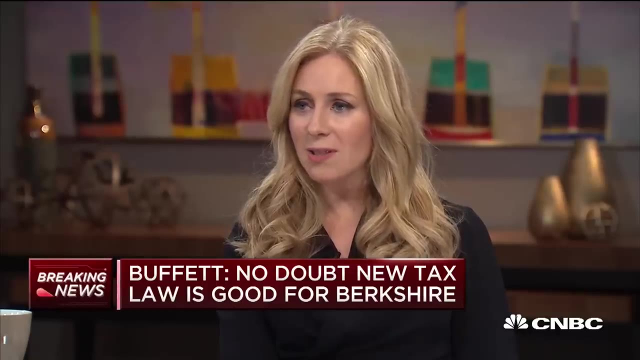 But I'm sure it's a very, very high. percentage of his net worth is in Berkshire Hathaway Energy, And it pays no dividend, incidentally, And Berkshire itself owns 90% of it. So our interests are very aligned. And, by the way, you don't hand out stock options. 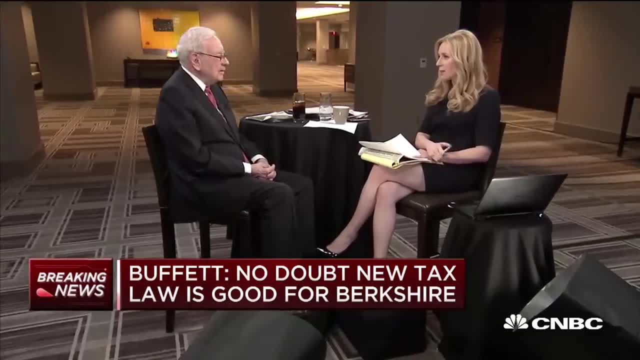 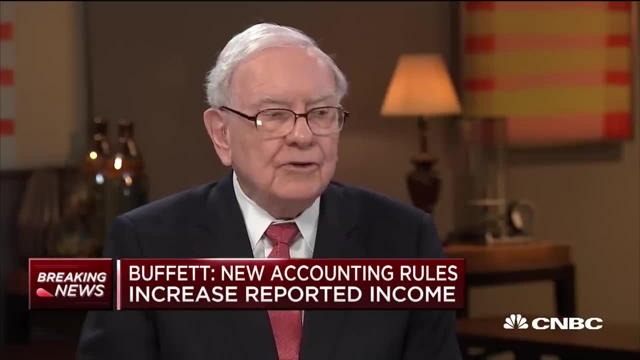 Like a lot of companies do. These are sums that they've kind of built up themselves over the years. Ajit has bought every share of that in the open market And he buys it just like anybody else. If it goes down, he suffers. 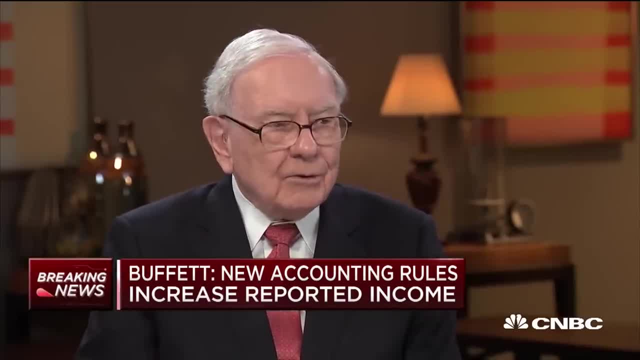 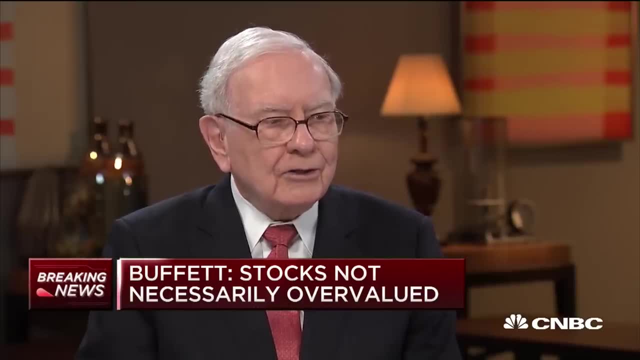 I mean we do not have one-way things And we don't grant the directors restricted shares or anything of the sort. We want our directors to stand in the shoes of the shareholders. We don't have directors and officers insurance liability. I think maybe one other company on there- 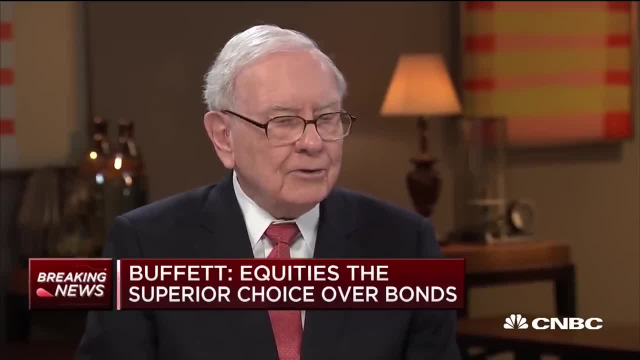 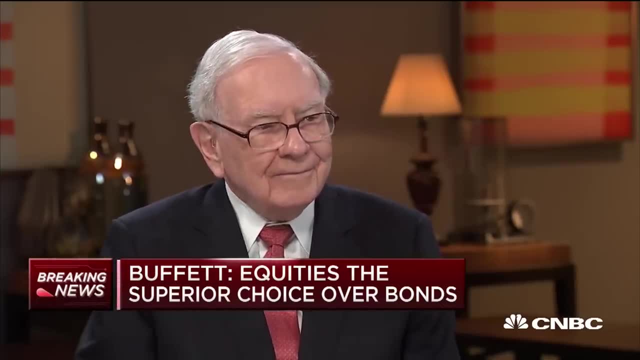 If we do something really dumb and the company loses a lot of money. they lose money and it's real money to them. It isn't just something that was given to them. You didn't know how much either of them owned before, did you? 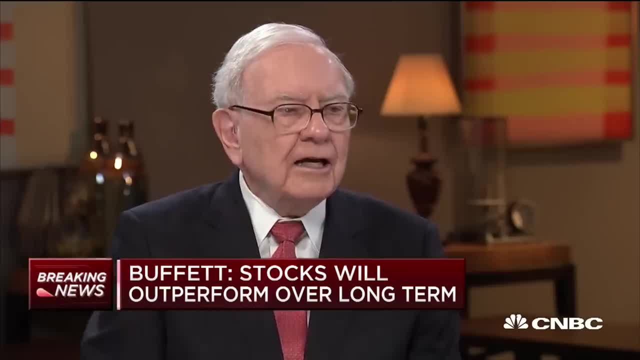 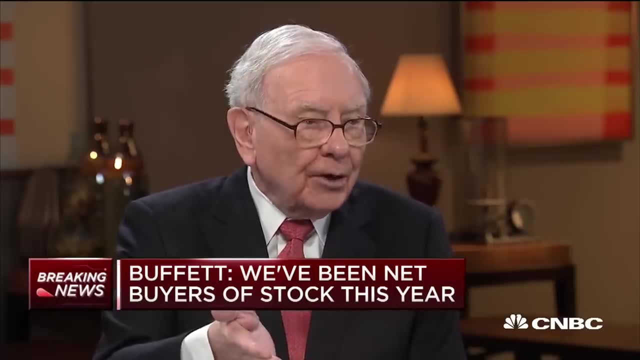 Well, I knew how much Greg owned of Berkshire Hathaway Energy. I had no idea what his holdings were of Berkshire And I didn't know. I mean, I knew Ajit owned it, but I had no idea what the amount was. 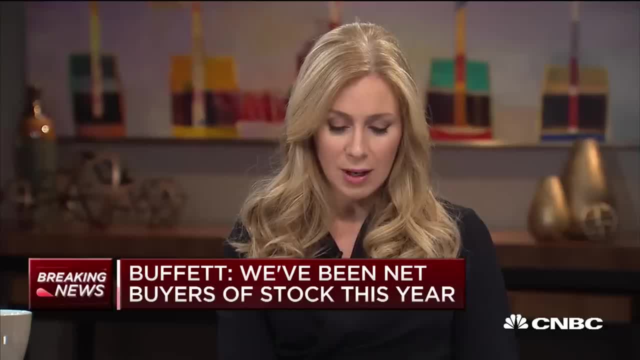 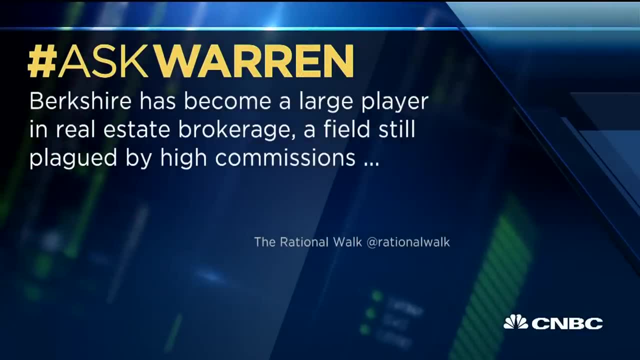 Here's another question that comes in. This one's from The Rational. It says Berkshire has become a large player in the real estate brokerage, a field that's still plagued by high commissions. I recently sold a home using Redfin and saved at least 2% of commissions relative to traditional brokers. 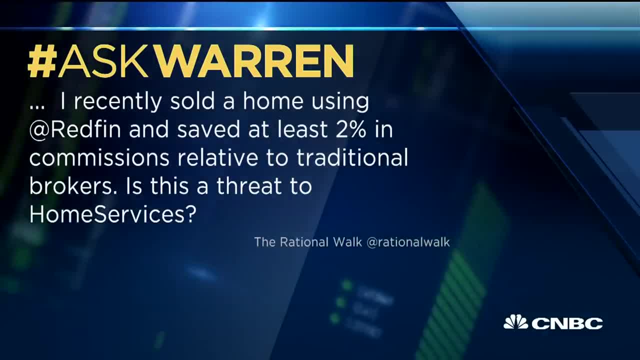 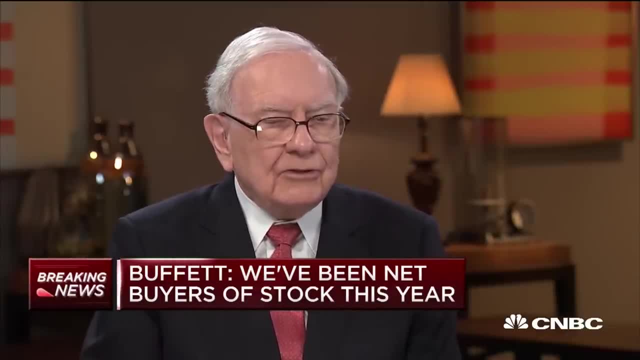 Is this a threat to home services? Yeah, I don't think it's much, but I could misjudge that. But obviously the Internet's going to try and take away any business that existed in a more traditional form in the past. Buying a home is the biggest deal that most people make. 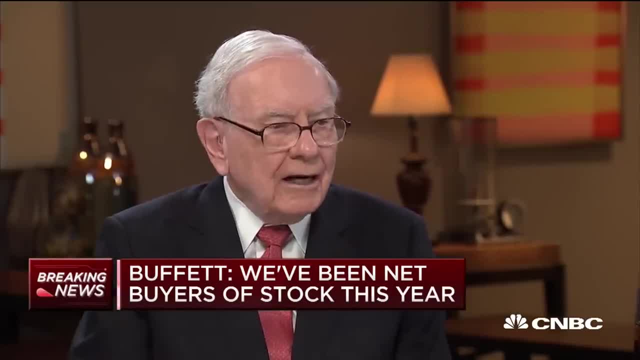 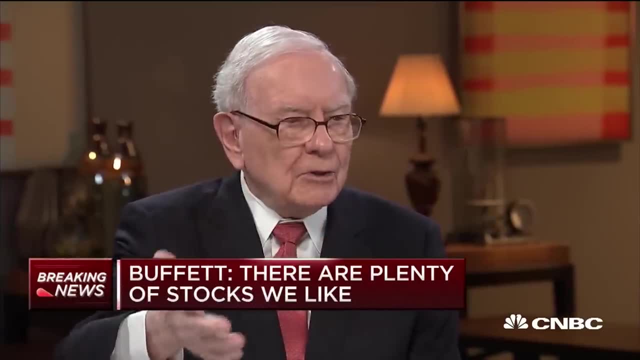 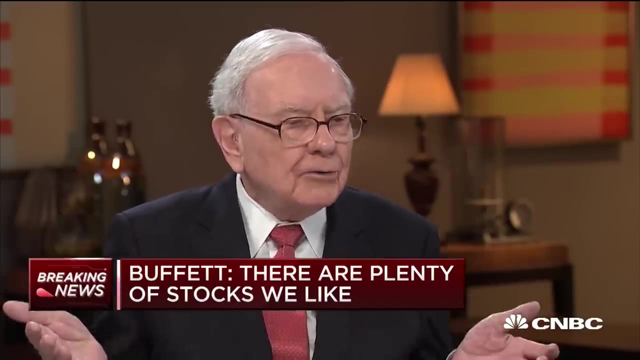 It's the biggest deal that's ever happened in their lives. Sometimes they're moving from another city and they want somebody that explains the schools to them and just how the whole city works. They really want a helping hand in coming in and it's a very personal transaction. 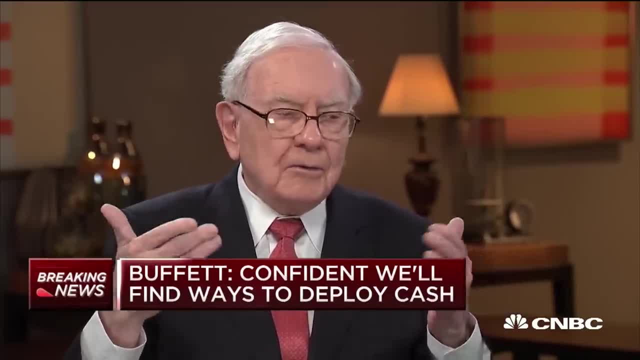 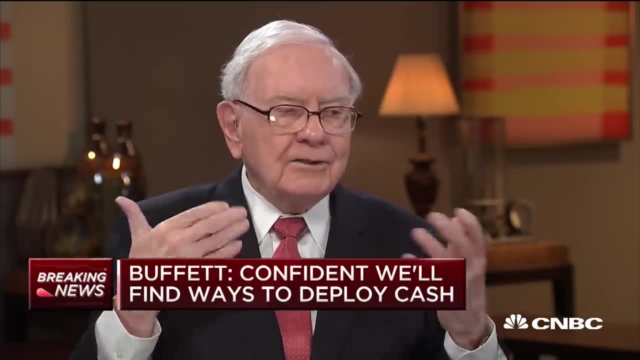 It's a scary transaction sometimes to people, a lot of paperwork involved and all that. They really want somebody they trust, And I have a feeling that it will be very much a person-to-person operation 10 or 20 years from now. But the people who are backing an Internet operation think otherwise. 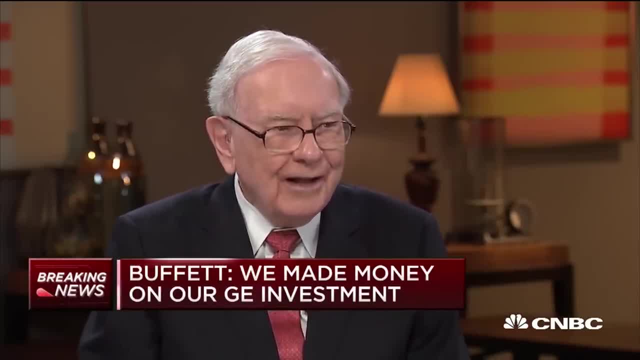 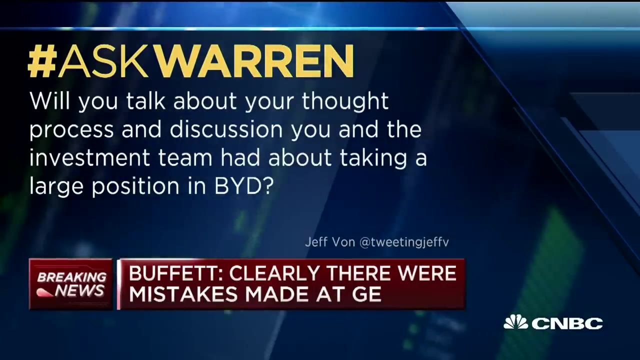 And certainly Amazon has proved that a lot of businesses that you thought had to be done face-to-face can be done very well from thousands of miles away. This question comes in from Jeff Vaughn. He says: Warren, will you talk about your thought process and discussion that you and the investment team had about taking a large position in BYD? 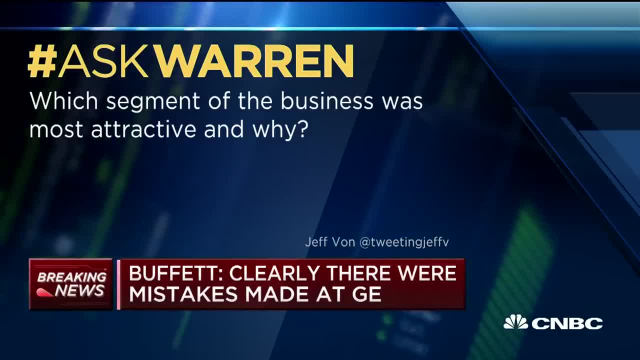 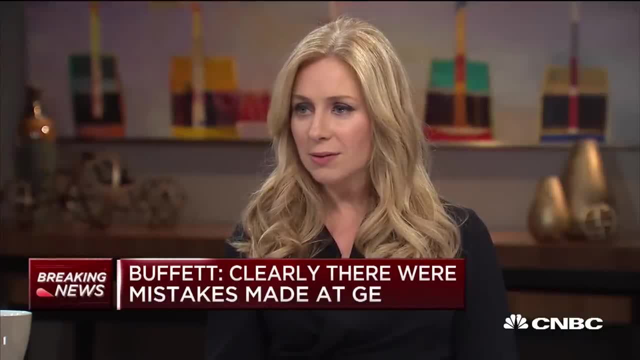 Which segment of the business was most attractive And why. And that comes up because BYD made its way into the top 15 holdings of Berkshire again this time around. Well, I've said in the past, it really wasn't me or the investment team. 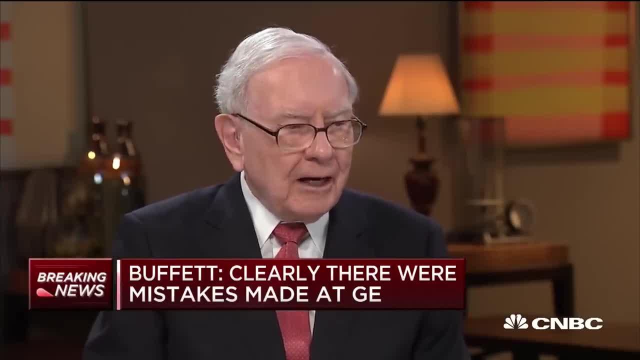 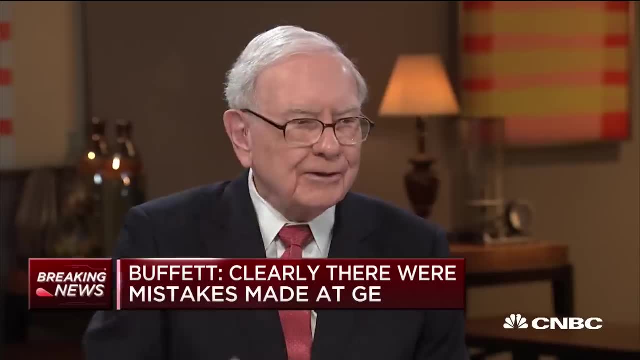 Charlie called me one day and says we've got to buy BYD. This guy that runs it is better than Thomas Edison. And I said that isn't good enough. And then he called me later and said he's a combination of Edison and Bill Gates. 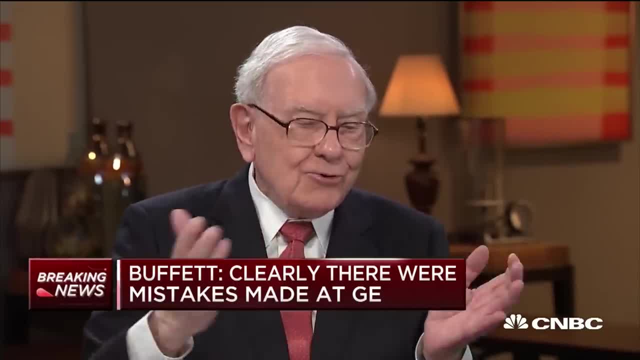 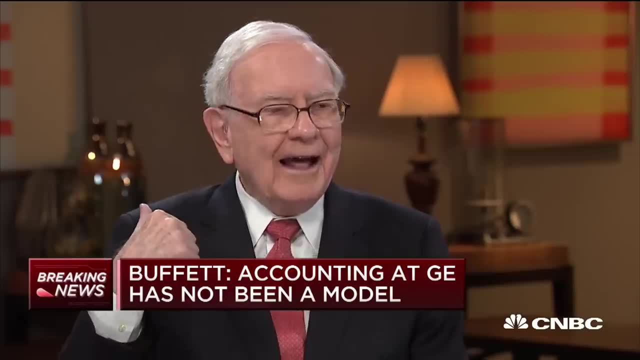 I said: well, you're warming up, but it still isn't good enough. Anyway, Charlie wanted to do it. Now it's worked out so well. I'm actually starting to remember that it was my idea. It's coming back to me. 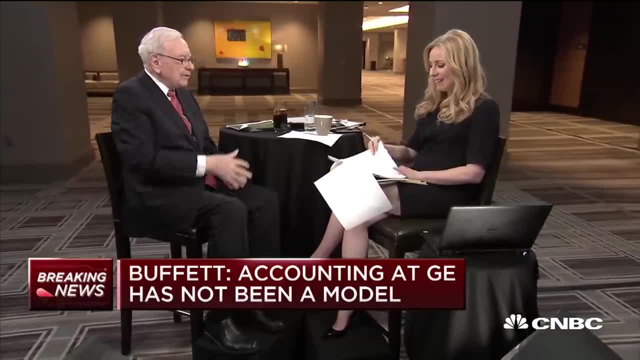 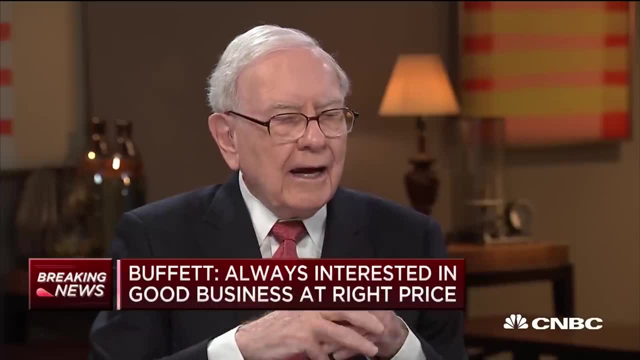 I think I persuaded Charlie, But unfortunately I'm on the record that it's his deal. But BYD, Charlie's in love with the company And it's done very well And with all that runs it. you know, there's autos and batteries. 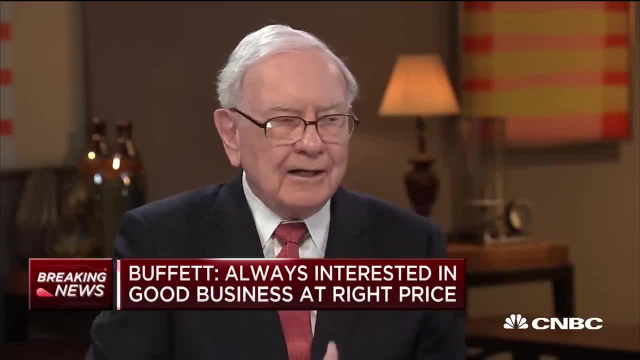 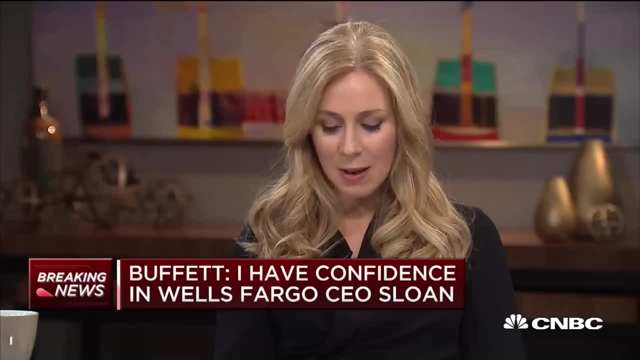 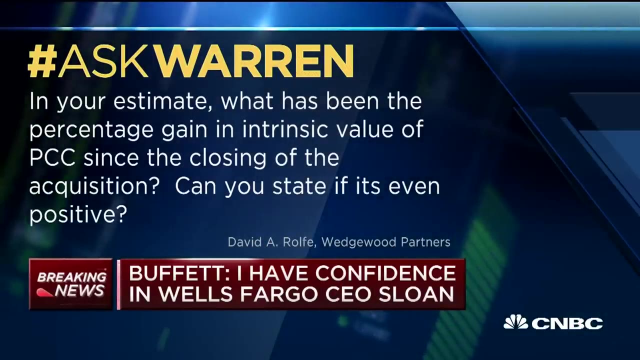 But he's got big, big ideas And he's very good at executing. But I leave it to Charlie. There's another question that came in from David Wolf And he's asking about precision cast parts. He says: what's the percentage gain in intrinsic value of PCC since the closing of the acquisition? 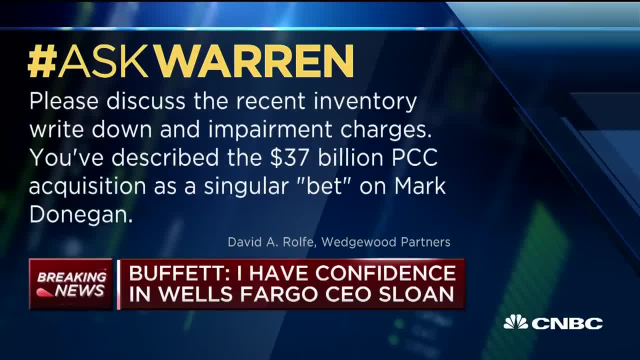 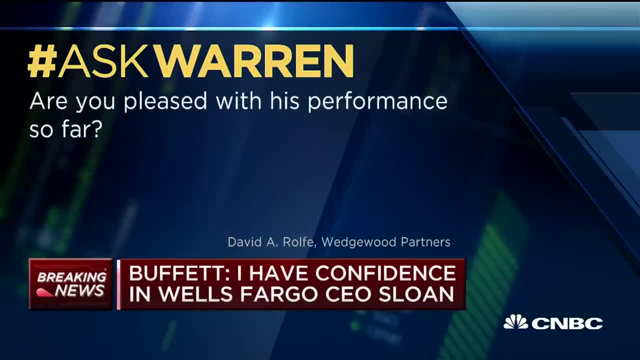 Can you state it? if it's even positive, You've described the $37 billion PCC acquisition as a singular bet on Mark Donegan. Are you pleased with his performance so far? Yeah, I am, But it has not earned as much as was in the projections. 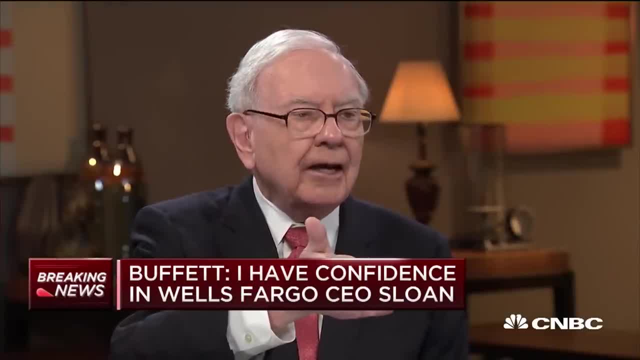 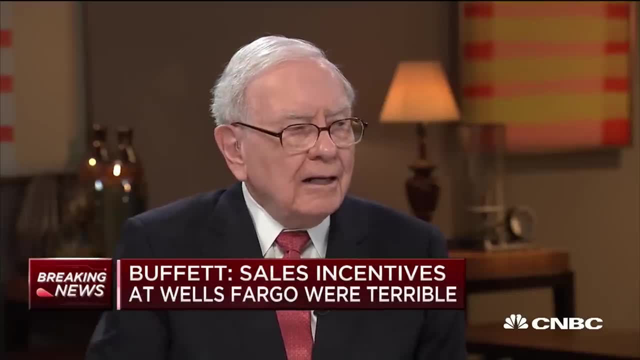 But that's a very long-term business And the contracts they've made- they've made The contracts they get- can run out into the mid-2020s. And Mark- I just saw him about two days ago And he is an extraordinary business operator. 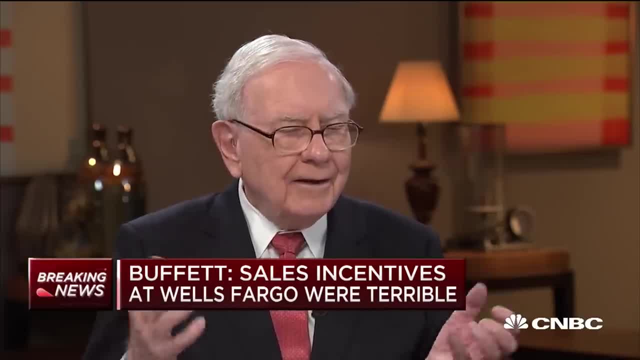 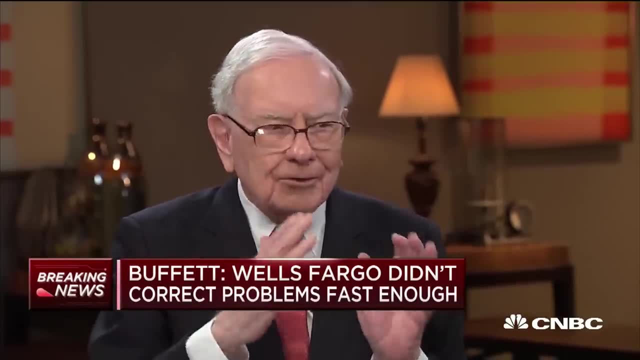 I mean, he just loves figuring out how to make things And he hits it off perfectly well with our fellow who runs his car, Because they've got that kind of mind And they're very, very good at it. And Mark never stops working. 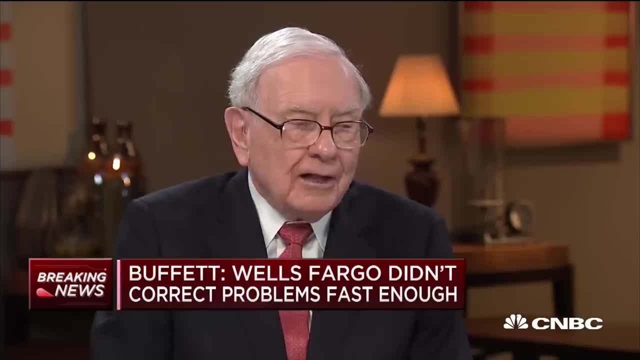 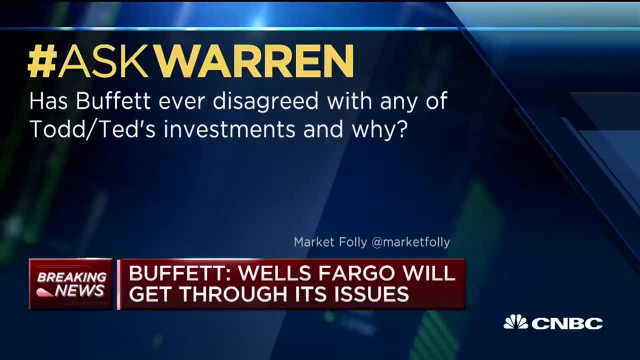 And he built a sensational company And he will continue that with us. And finally, Market Folly writes in about the relationship with Todd and Ted, the investment gurus in-house. He says: has Buffett ever disagreed with any of Todd or Ted's investments, and why? 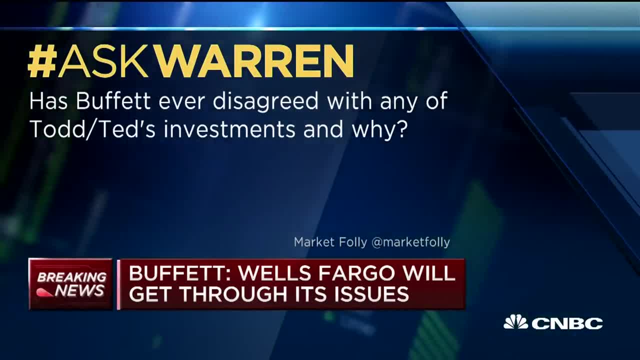 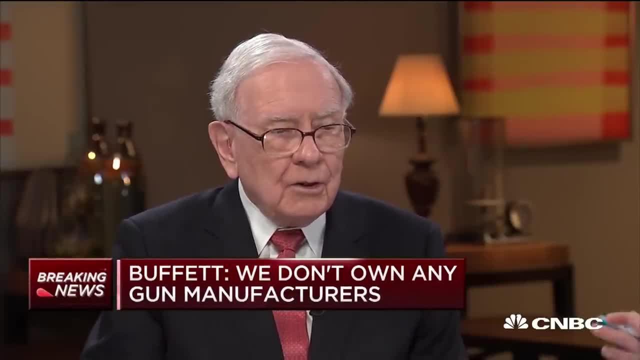 Well, they make their own decisions 100% And they each manage $12 or $13 billion. now, It started as: what about $5 billion each? Pardon me, They started out with each of them at $5 to $6?. 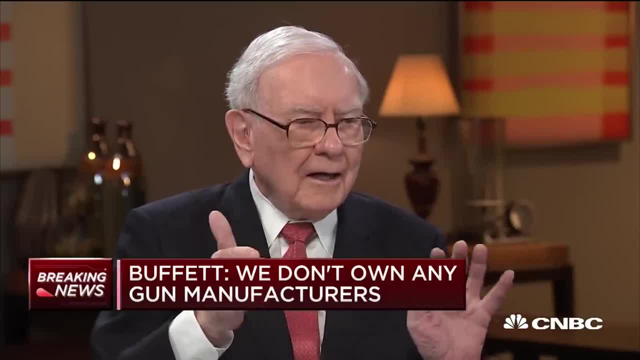 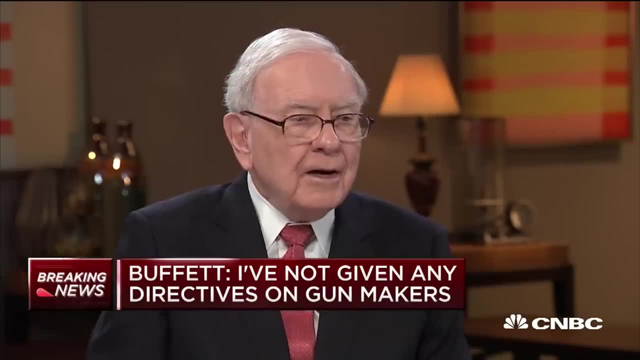 Actually, I think when Todd came about a year ahead of Ted, And I think maybe it was $2 billion then, But it has increased at various points And then they've earned a lot of money- Fort Berkshire, which builds up for them too. 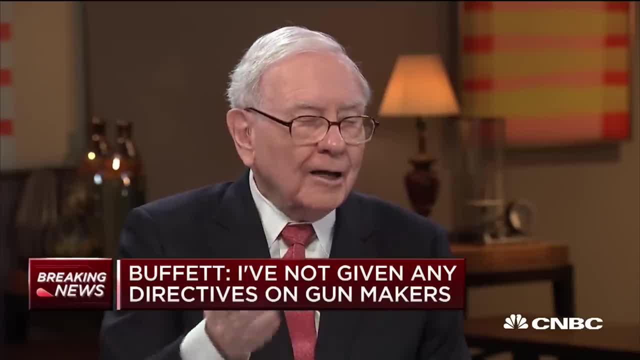 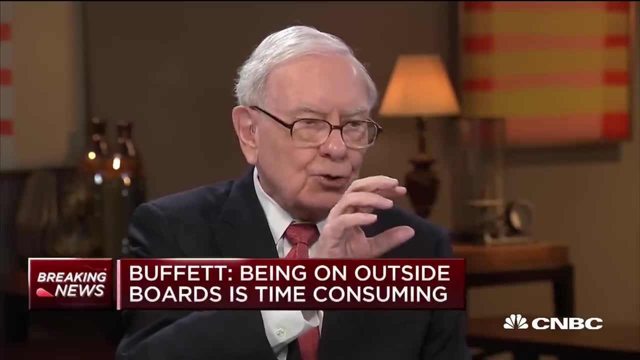 Certainly they've done things I wouldn't have done, But I've done things they wouldn't do too. I mean, I want them to figure out their own choices. They are good at managing money, And they've got the advantage of managing smaller sums. 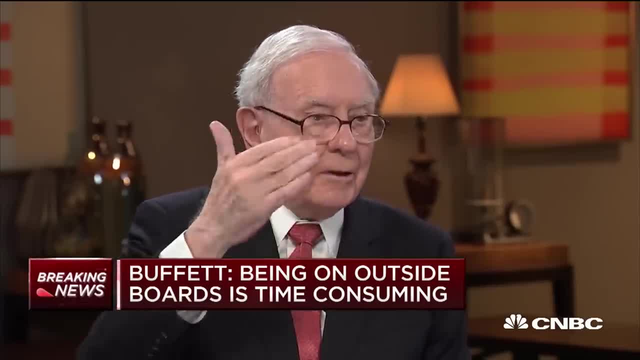 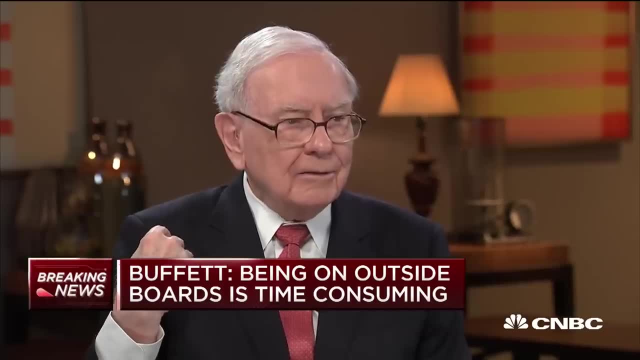 Then I'm running. But they've got the disadvantage of running quite a bit larger sums than most people run. I mean, it gets more difficult with size. But they not only have done a good job of managing the money and trusted them, but they've contributed to Berkshire in just dozens of ways. 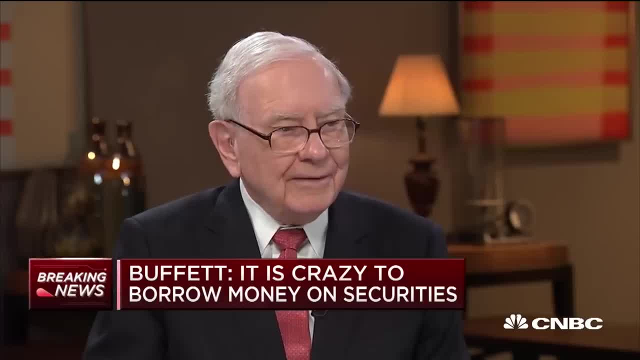 They were sensational hires. Do you talk about the investments with them ahead of time? No, not ahead of time. And there's a number of them. I haven't talked with them at all. I couldn't even Name three quarters of their portfolio. 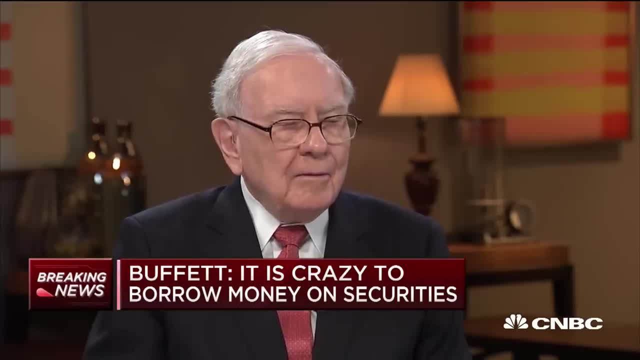 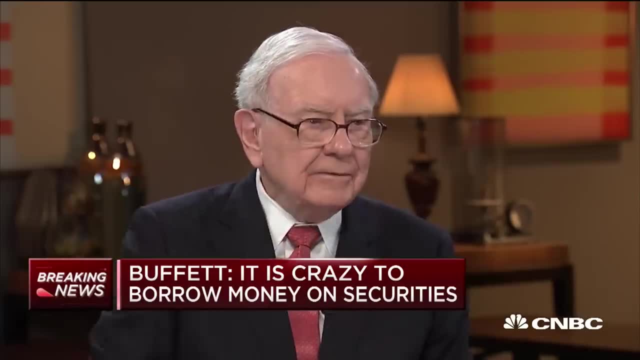 I couldn't tell you the amounts, I don't remember that well. But I've gotten ideas from them. But they take on other tasks. I mean, Todd is on the health care situation. He's there on Saturday. I was there on Saturday. 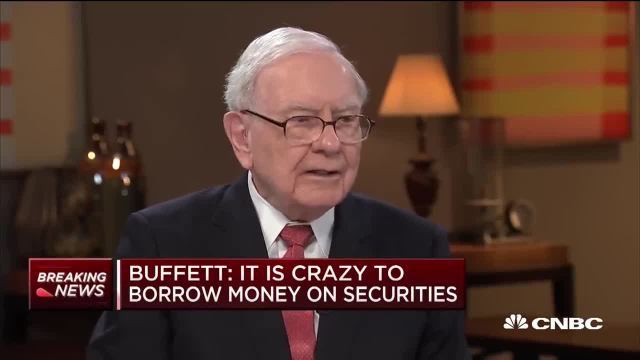 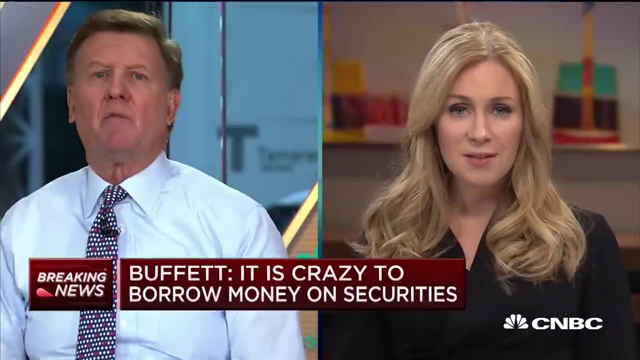 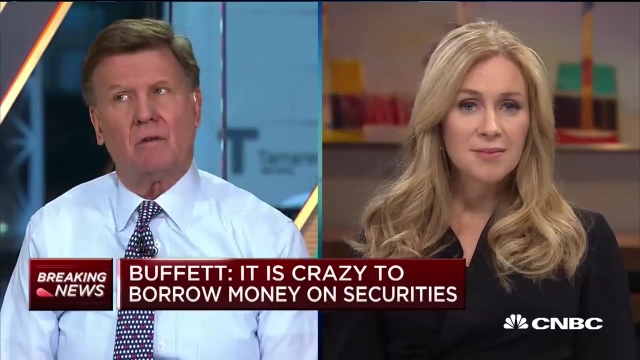 He's there all day talking to people around the country in terms of looking for the right CEO and that sort of thing. They are enormous contributors to Berkshire- Some of the most pressing social issues facing us. Becky, Do you know whether he's a Taco Bell or a Chipotle guy? 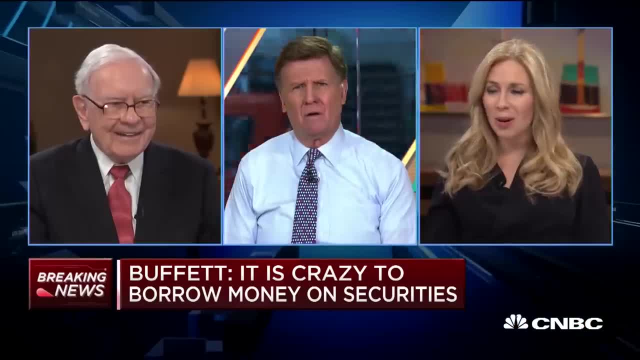 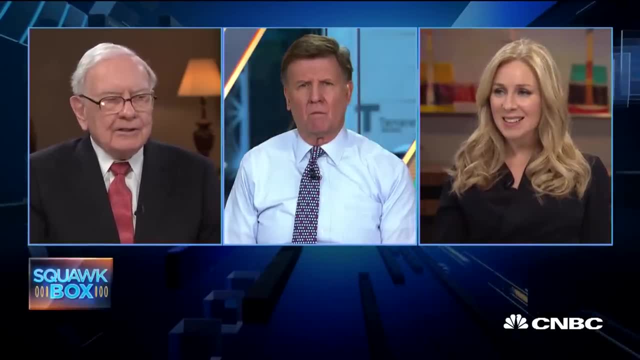 Have you ever asked him? I'd have a guess. I don't know. Have you been to Taco Bell or Chipotle? Neither one, Neither, Neither one. No, I go to Kentucky Fried, I go to McDonald's. I go to Burger King. 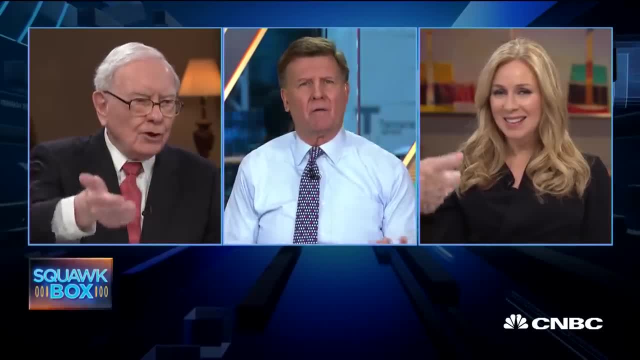 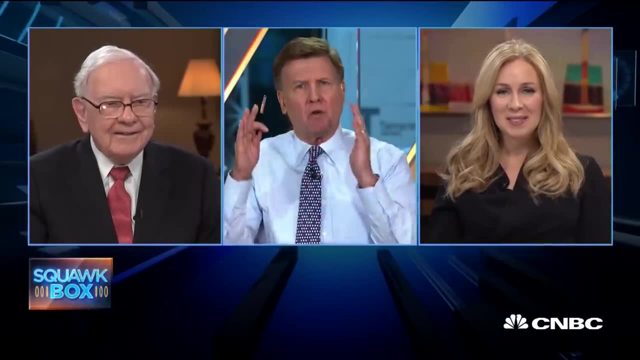 We go to Wendy's. You're skirting the question And there's various local ones Skirting the question. Taco Bell, Will the Taco Bell guy be good at Chipotle or will he ruin the natural foo-foo? you know all the. you know I mean Taco Bell. 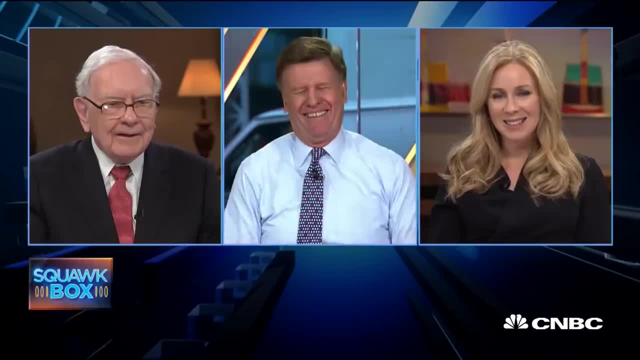 Knowing his inclinations for where he's he just I don't think he's a Taco Bell guy. When they start serving hamburgers, I'll give you an opinion. Yeah, I don't think he's a Taco guy, All right. 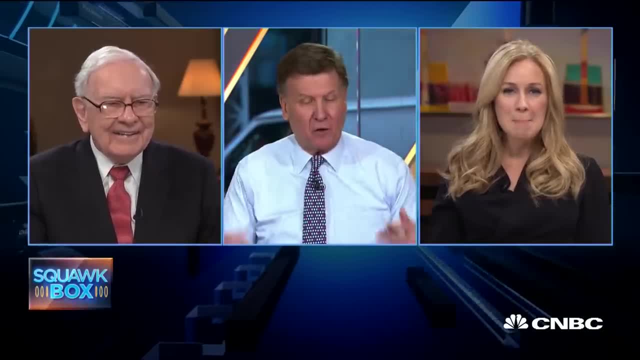 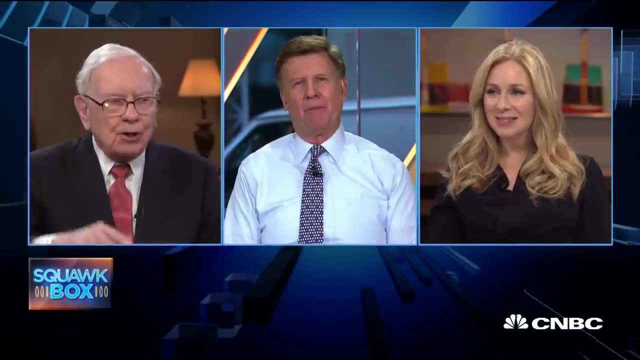 All right, I was just. these are the pressing. you know, these are what's on my mind. As I said, I wanted to prepare you for some of these social, societal questions, Big questions: Everyone serves Coca-Cola. I'm actually just looking at this. 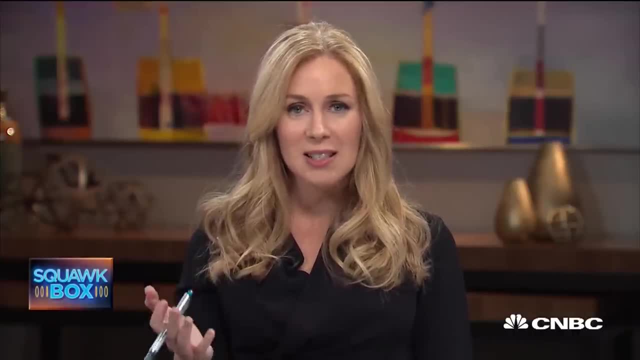 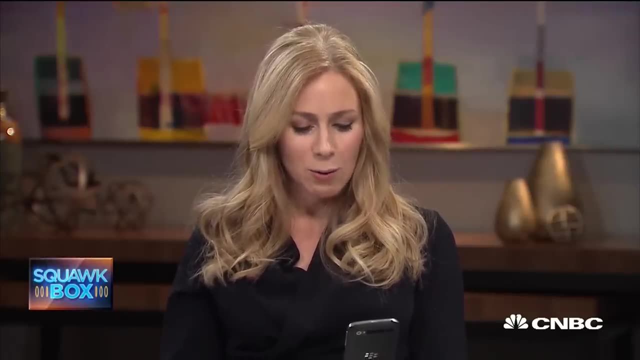 Well, no, I was just showing him, I was laughing. You know I've been watching the wires to see what he says, makes the wires And literally Joe, this honestly just hit the wires At 744 and 48 seconds. AM Buffett says has not gone to Taco Bell. Chipotle prefers McDonald's, KFC, Burger King, Wendy's. 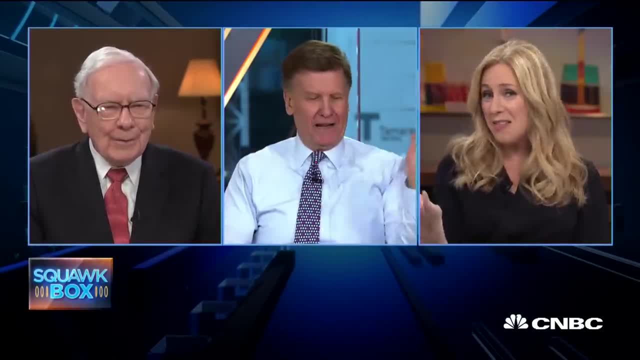 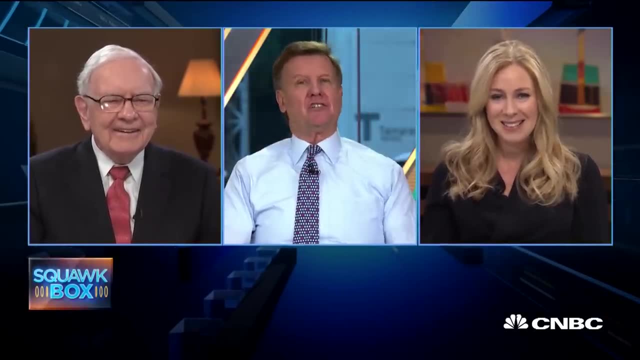 I'm not joking. That literally hit the wires. I'm getting Twitter, So I think he can say anything. Yeah, 85-inch screen Within, literally, within Exactly Within milliseconds. Drudge had Buffett touts tax plan. They had that. 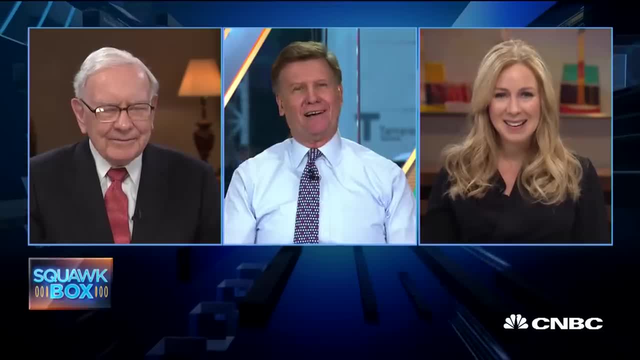 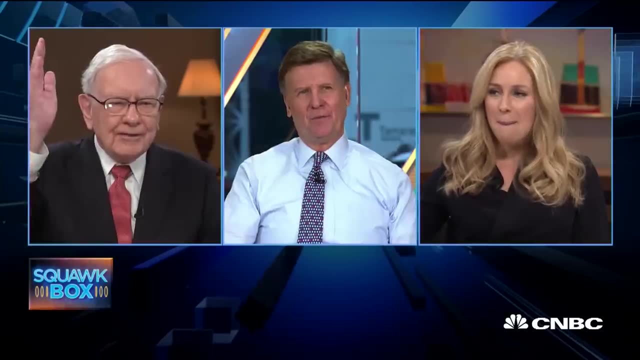 I thought I was going to be the lead there, but that got on Drudge almost immediately too. So let me check Huffington Post, But it's not nearly as important as this comment that just made the wire: You too can live to 87.. 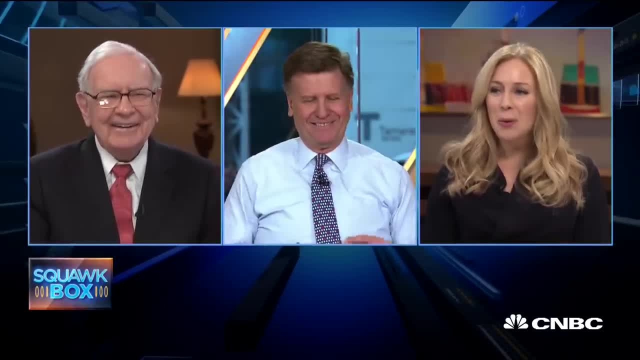 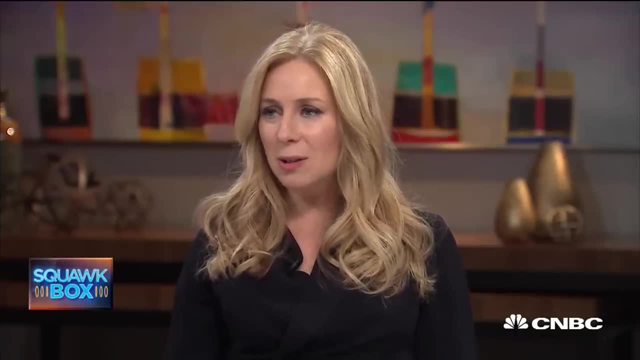 Yeah, exactly That'll come out, Warren. one thing that you said earlier: you were talking about Samsung. You mentioned, you know, the Samsung 85-inch television screen, But you know an awful lot about the company. You don't own the shares, do you? 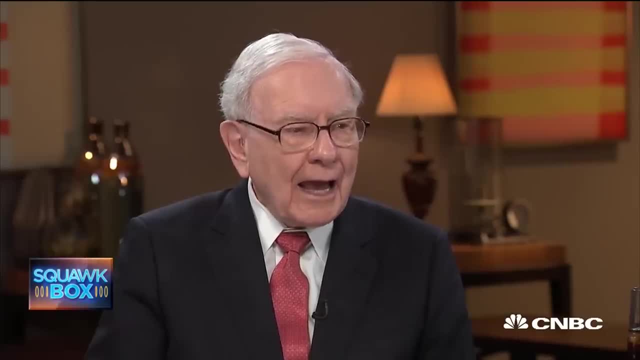 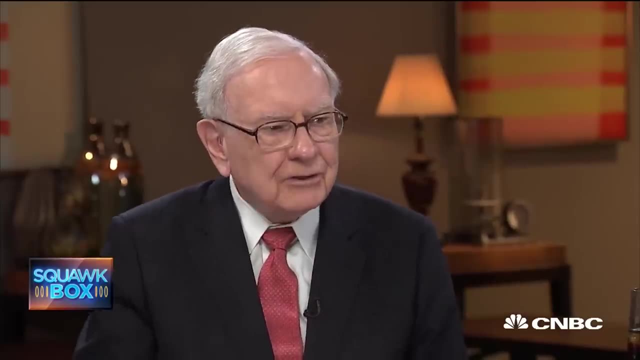 I don't own them and Berkshire doesn't own them now, But Berkshire has owned Samsung. It doesn't get reported in our 13F- I think 13Fs just apply to domestic, So it actually hasn't shown up. But I think I'm right on that. 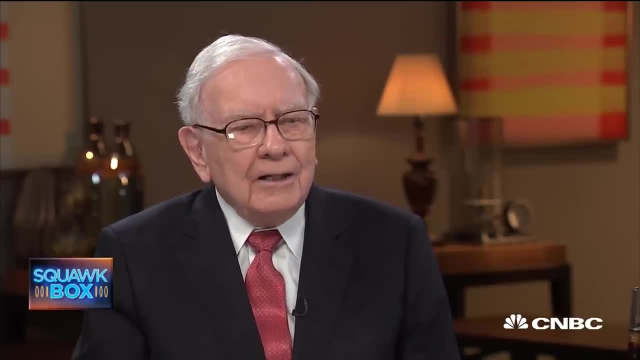 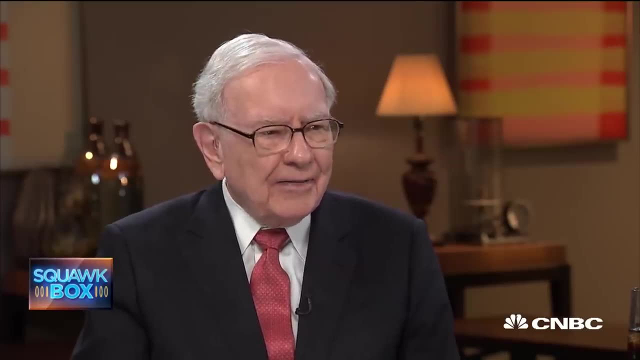 I'm 99% sure, And so we bought some When Samsung was at about a million won. You've got to divide that by something over 1,000.. We bought a reasonable amount. We did sell it when it went up. It's higher than it is now. It went up to 1.8 million or something. I think it's around 2 million, 3 or 4.. The won went in our favor a little bit too, So we did a little bit better in dollars. 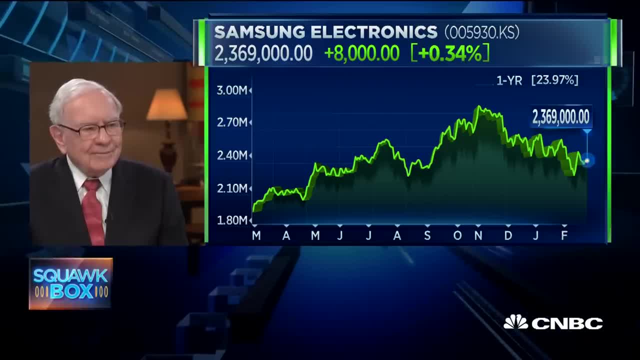 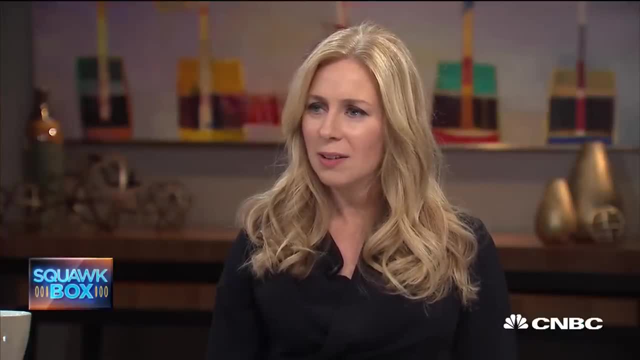 I mean, I don't think of you as – in the past, you have bought some South Korean stocks. I think That was a while ago. Why? Why were you looking at Samsung at this point? It was very, very cheap. They had a lot of cash. 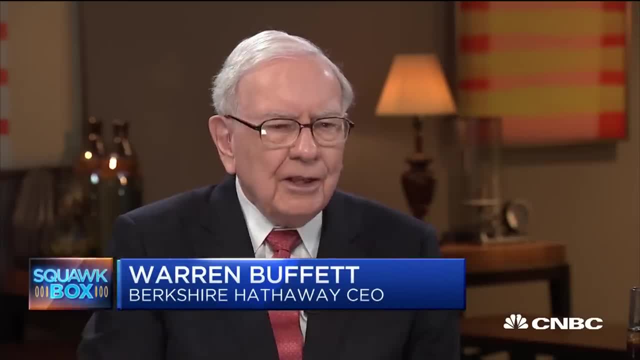 They hadn't done much on buying in their stock but they had talked about it, But it was just very cheap. It was a big, strong, good company. Yeah, I remember you buying a South Korean retailer, Was it years ago? 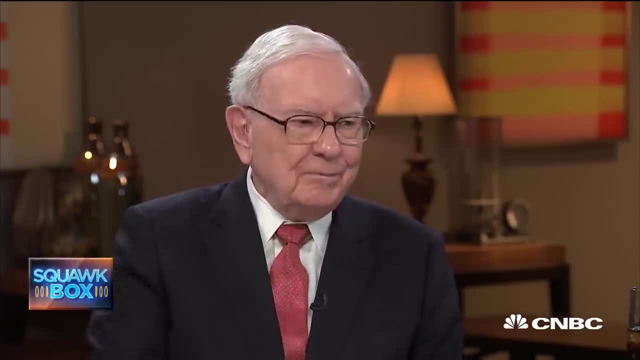 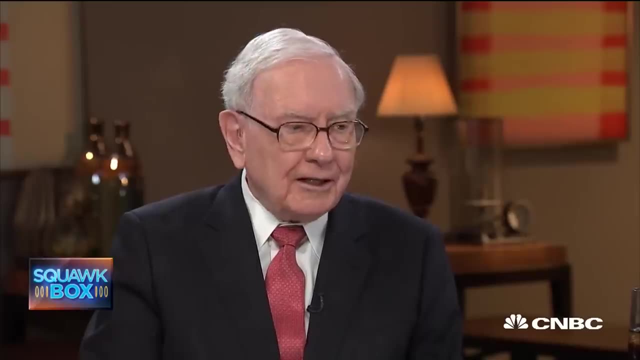 Yeah, There was a time when I bought a whole bunch of little ones, Right, right about the time when we traveled. Yeah, exactly, The Korean market was very cheap. I mean ridiculously cheap After the 1998, when they had all kinds of troubles. 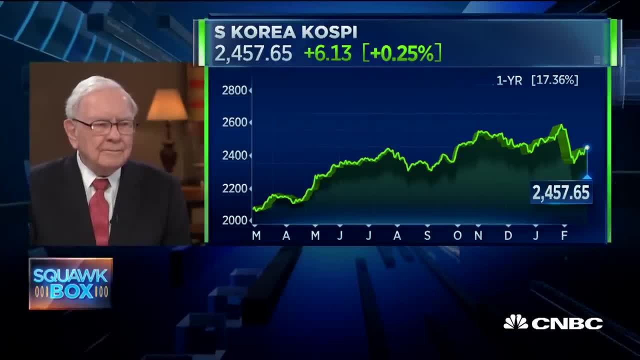 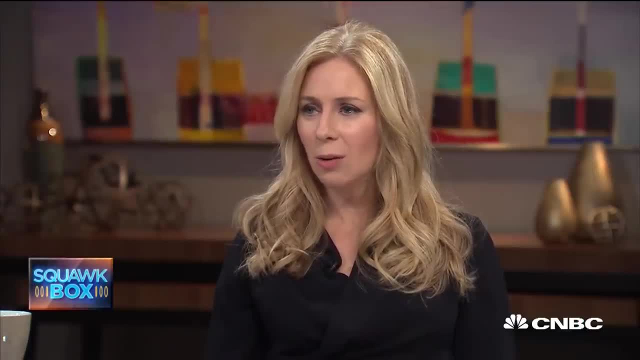 And there were a lot of bargains in Korea. When you say a reasonable amount, I mean for me. that's a different number for my holdings than it would be for you. Yeah, Are we talking north of a billion dollars? Well, we probably made in the hundreds of millions someplace. You made that much on the transaction. Yeah, That's my memory. It would have kind of been 500 million or 400 million, I don't remember exactly. Let's talk about some of the other purchases that were revealed, Purchases and sales that were revealed in some of these most recent filings, the 13 Fs. 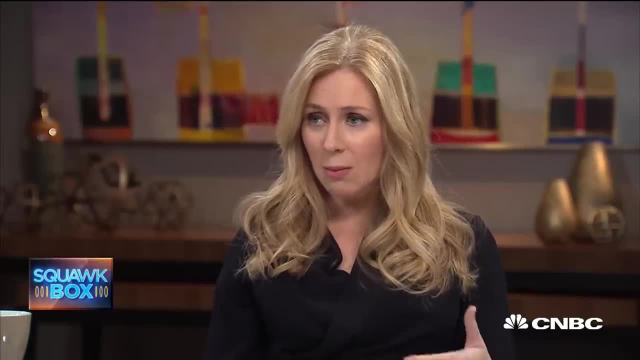 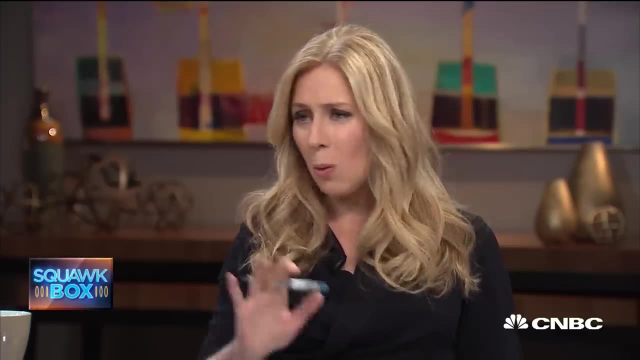 You sold more of your IBM stake and bought more Apple. according to the latest filings that we had seen, That's true, And a question came in from Brandon Carroll that said: first of all, why did you? Well, I was wrong on- at least I felt I was wrong on- IBM. 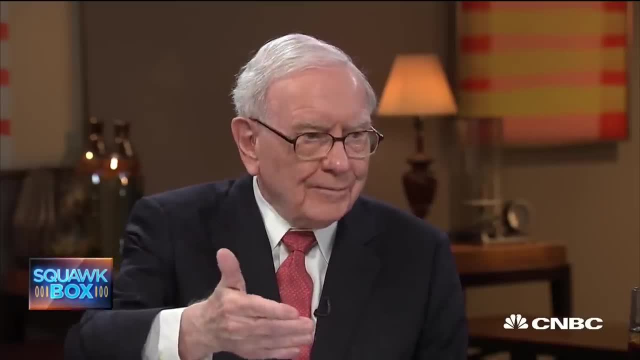 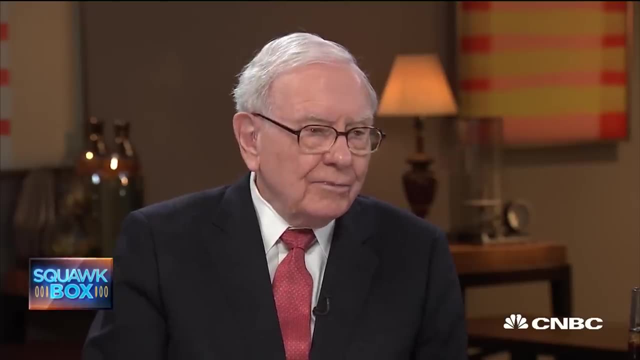 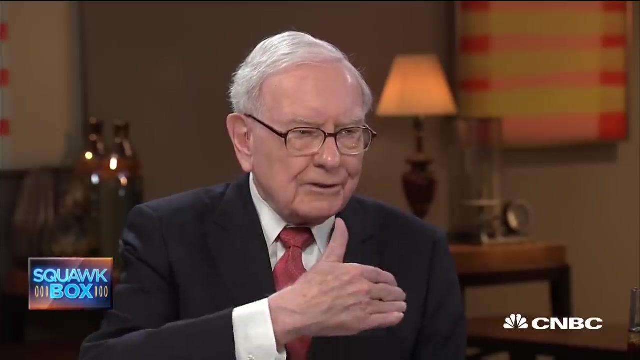 Now, I may have been wrong when I sold it to it, but I certainly was wrong when I bought it And I felt that Apple has an extraordinary consumer franchise. Apple's a different kind of business than IBM. They're both tech, obviously in a major way, and they even have a joint venture on some things. 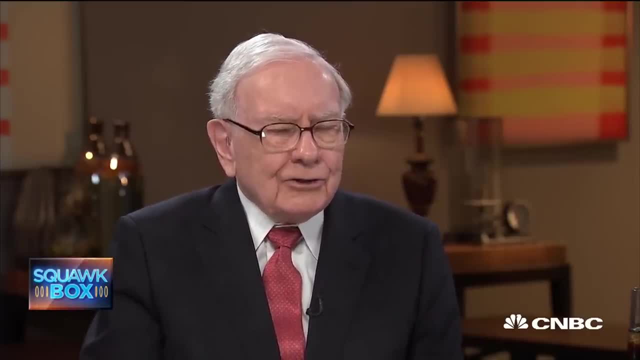 But I think I understand consumer behavior perhaps better than I do the tech business. It wouldn't take much to beat it. I liked it. I liked Tim Cook very much. I like their policies. I see how strong that ecosystem is to an extraordinary degree. 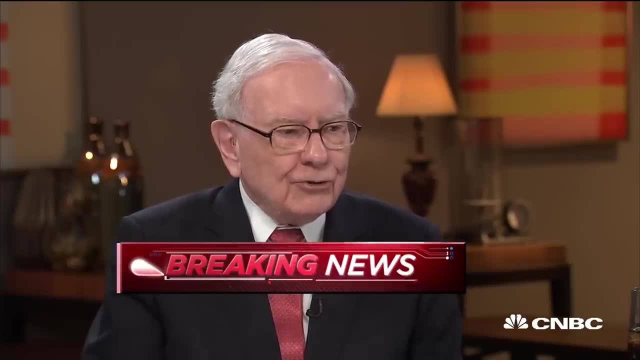 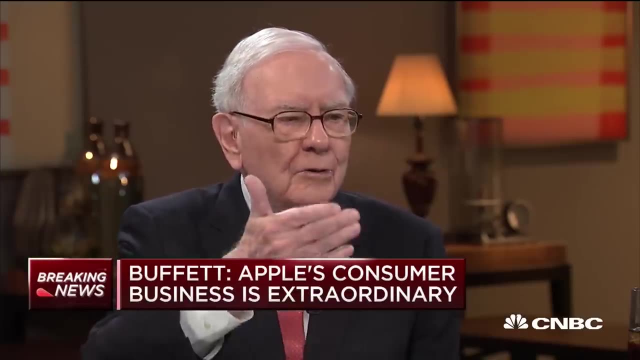 I mean I look at my grandchildren, my great-grandchildren and everybody in the office. I mean their families. I talk to the people at the furniture mart When the 10 hadn't arrived. nobody goes over to, you know, buy it. 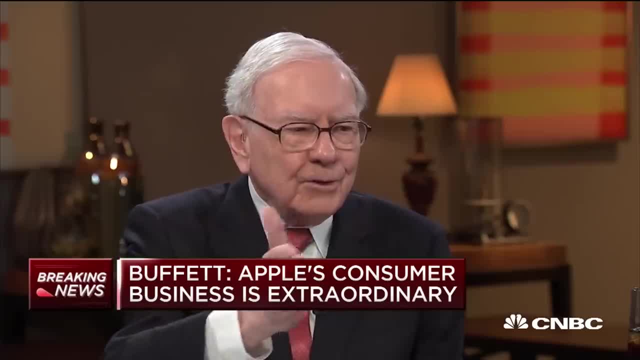 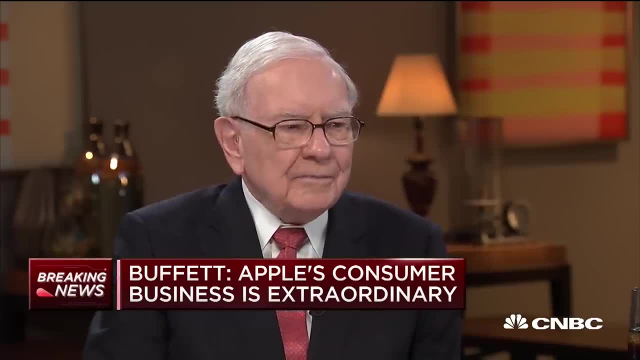 Buy it, Use that Android. I mean it's – you are very, very, very locked in, at least psychologically and mentally, to the product you are using. I mean you've got all kinds of stuff up on there. It is – it's a very sticky product. 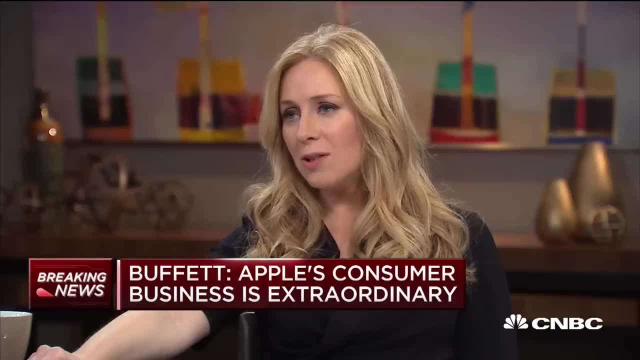 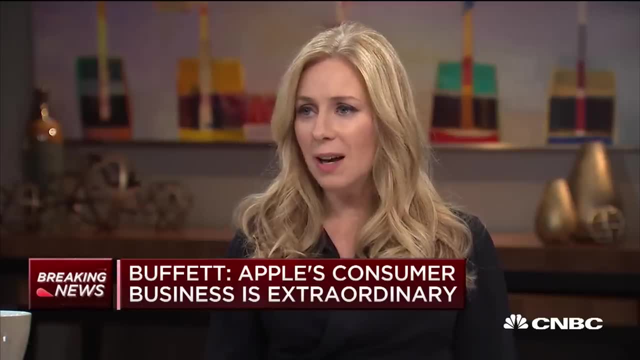 That was sort of the same thing you said about IBM when you were first buying it, That corporations that had bought into it they were kind of stuck with it That they – that it would be what they were using because it was too hard to get off of a system like that. 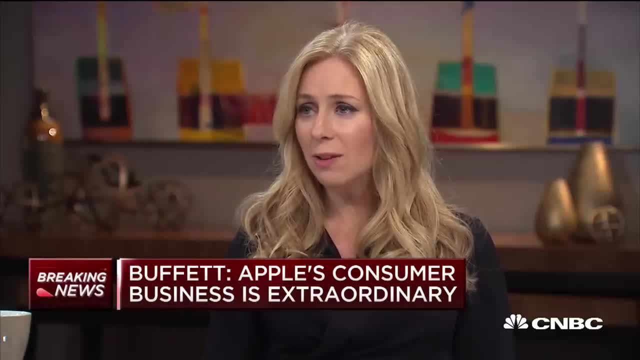 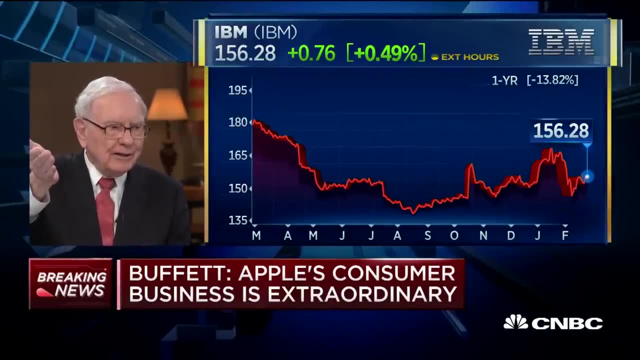 Yeah, IBM recently, just finally showed an increase in revenue for the first time in like 27 quarters, Yeah, but the foreign exchange went with them and it was the introduction of a new piece of hardware. I mean, actually they weren't up except for those two factors. 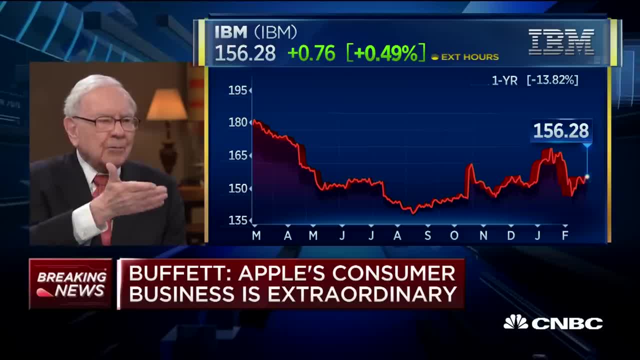 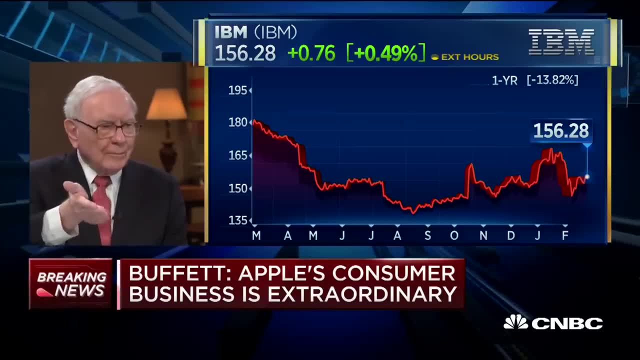 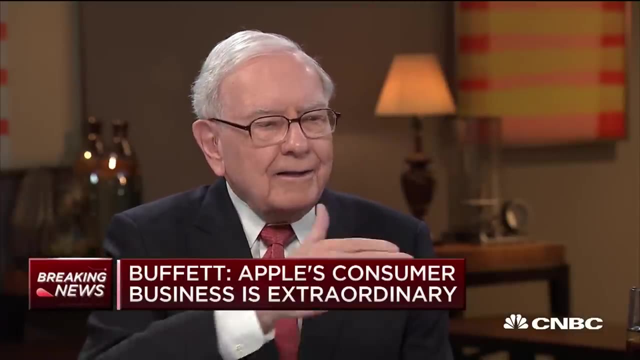 But the cloud came along and one of the most extraordinary things I've ever seen in business is when an unrelated type company, a retailer- you can call Amazon- of that type goes into another big industry and sees the future in it, gets into it. 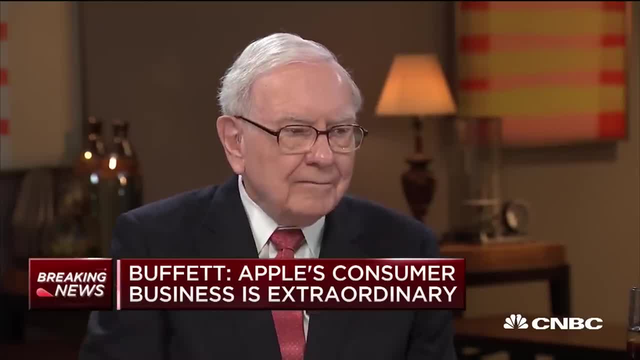 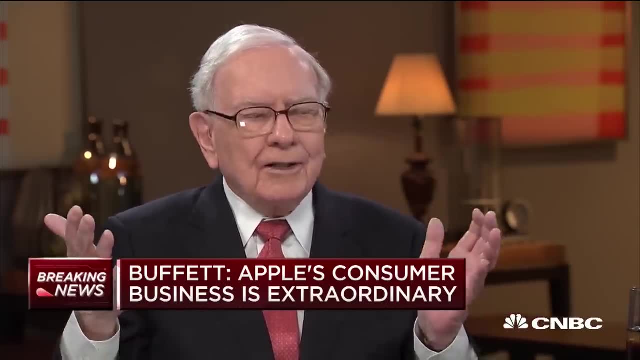 and then they gave, and Jeff Bezos would say this: he said it on the Charlie Rose show. he got this amazing runway. I mean, the other players here are all these 200 IQ people in that business- and they gave him year after year after year. 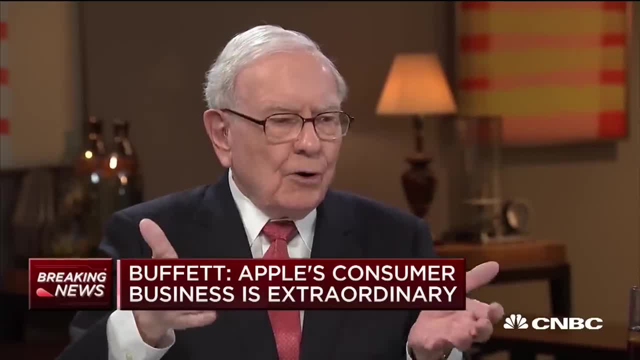 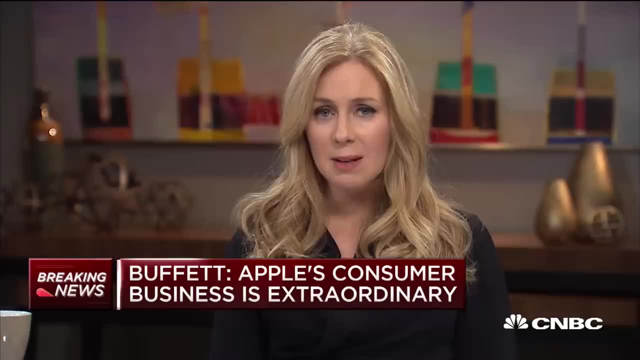 It wasn't a secret of what he was doing and he was, in an important way, revolutionizing. He was revolutionizing the industry and the other people sat on their hands basically, Wow, All right, we have more questions that we're going to ask you related to some of these things. 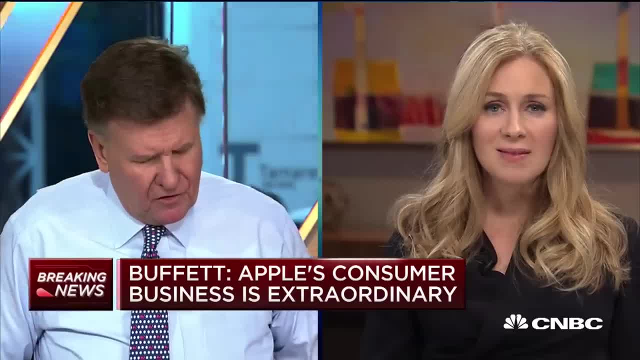 but right now we're going to send it back to Joe. Joe, Hold on, hold on. I just thought of something, Becky, Hey, Warren, I don't understand why Creighton's in the Big East. I don't know. 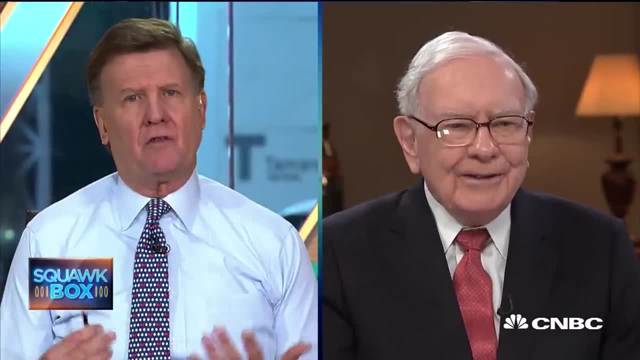 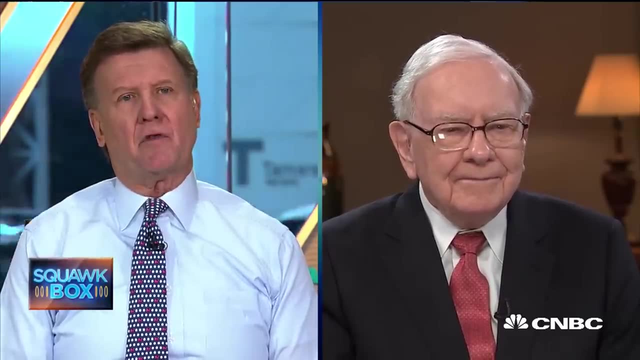 Number one because it's so far west. But let's just so it is. Why don't I'm inviting you? I'll get the tickets. You can come with my family. Why don't you come back for the Big East tournament? 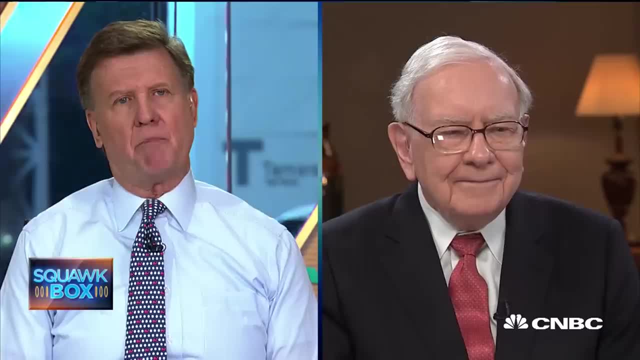 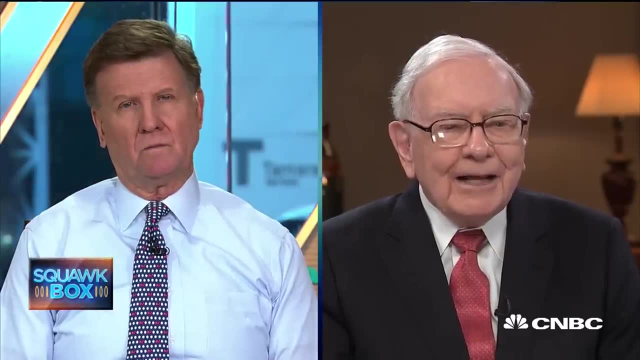 Not the March Madness, but it matters. Madison Square Garden. it's coming up the week of March 7th to 10th. You want to come back for that and we'll take in a couple of games. That's tempting, because I like watching Creighton basketball. 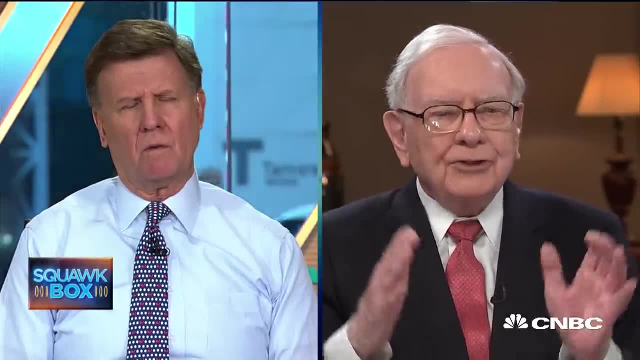 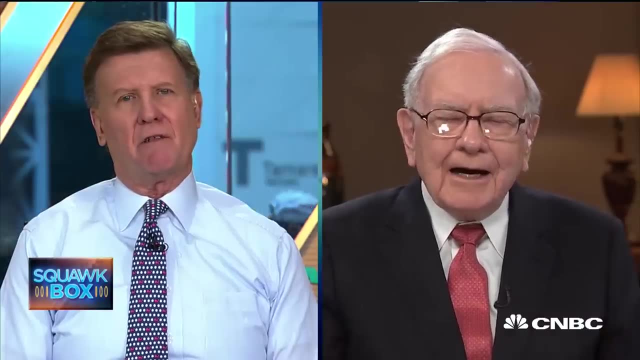 But I am cutting back on the travel. Joe, I'll watch it on my 85-inch. and you were talking about popcorn earlier. Now you're cutting back. I invite you somewhere and you're cutting back on your travel The minute. I invite you. to what? 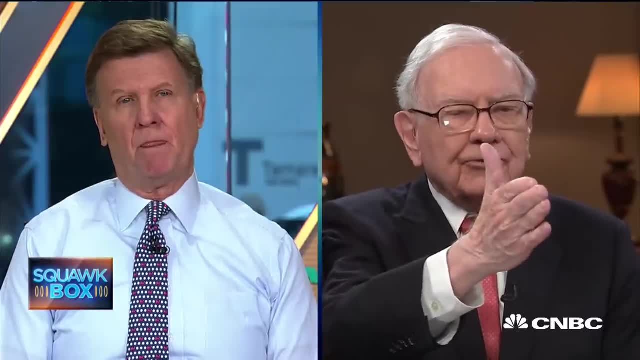 Well, I'll get good seats. I will. I'll tell you what I'll do. I'm making you an invitation. If Creighton gets to the finals in March, Madness, I'll take you. How's that? That's pretty good. 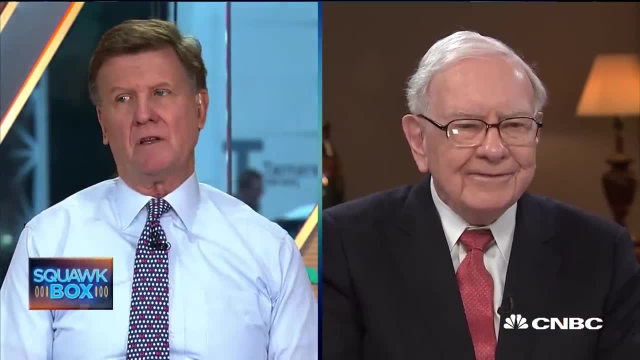 That's a firm offer, Because I'm not convinced they won't this year And I'll have good tickets. I'm not convinced they- I don't know who's good, You know. I mean there's a lot of everybody's great. 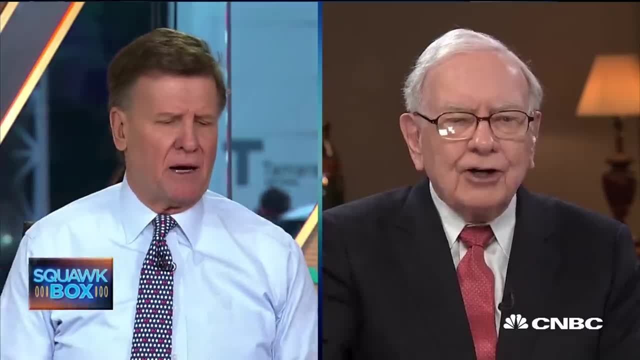 That's the thing, Amazing. All right, Okay, so forget it, Never mind. All right, good tickets, But you've got to be for the Blue Jays though. I mean, if we go, you cheer for the Blue Jays. 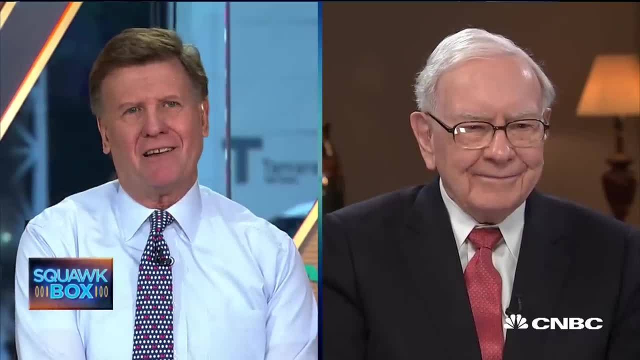 That's the deal. Not if it's against Xavier, I can't do that. Not if it's a Well, no, but All right. well, we'll see, All right. I just thought, because this is going to be. that's unbelievable. 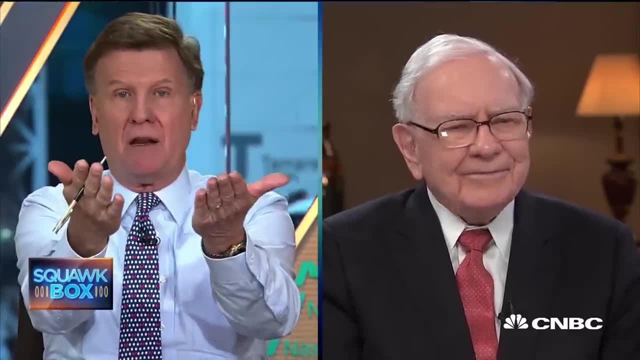 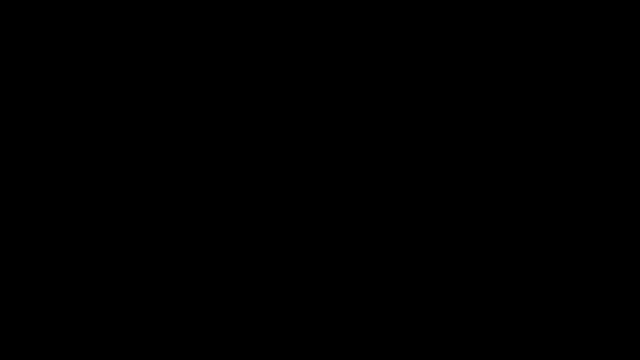 Madison Square Garden, that conference. I mean, if you can win in that conference, you can win anywhere, right? It's like the Southeastern Conference. Who would have thought it? Yeah, I know You're right. Hey there, thanks for checking out CNBC on YouTube. 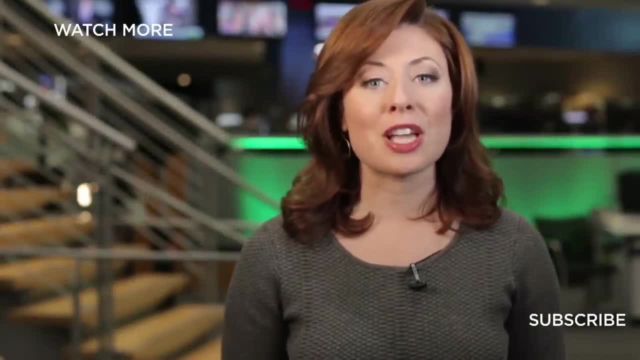 Be sure to subscribe to stay up to date on all of the day's biggest stories. You can also click on any of the videos around me to watch the latest from CNBC. Thanks for watching.